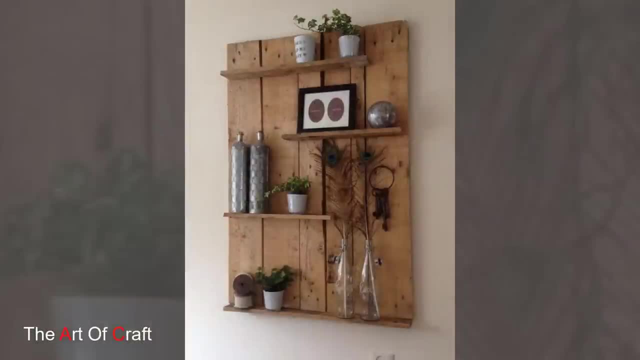 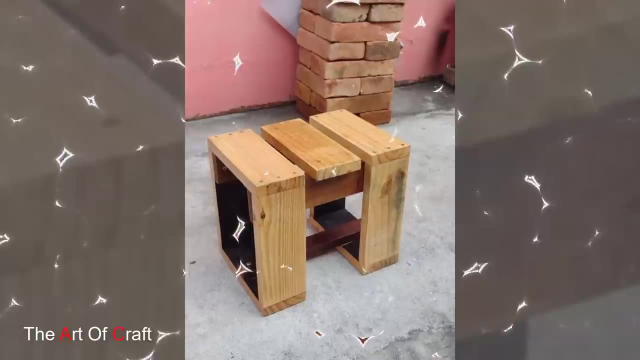 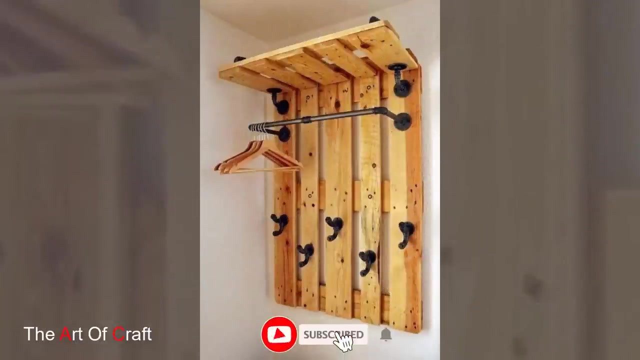 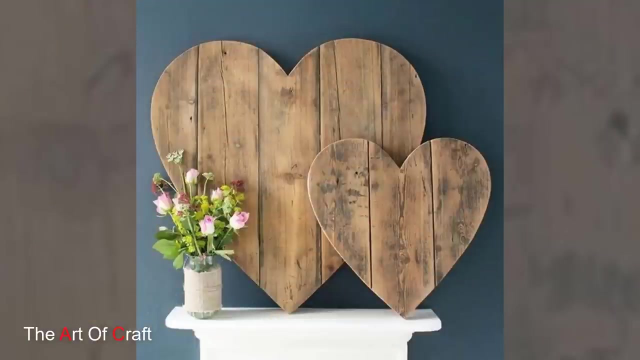 conscious of their environmental impact. The allure of sustainability and eco-friendly options continues to grow. Pallet furniture is not just about functionality, it is also an art form. Skilled craftsmen and the other enthusiasts alike revel in the creative freedom this business offers. 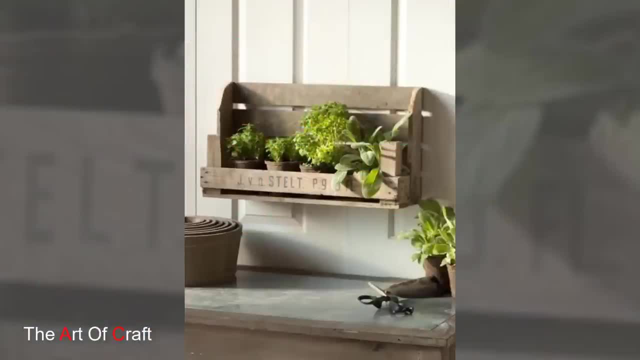 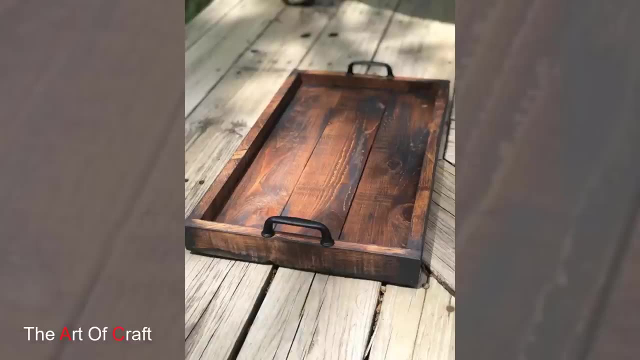 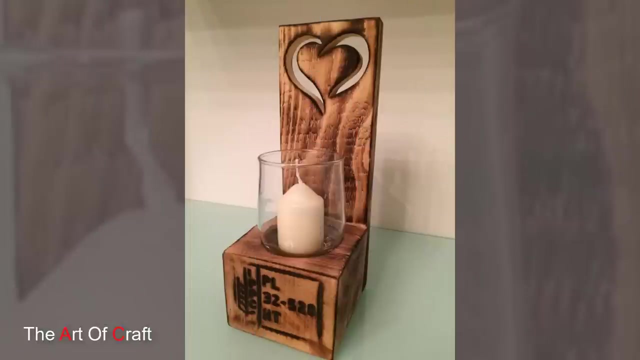 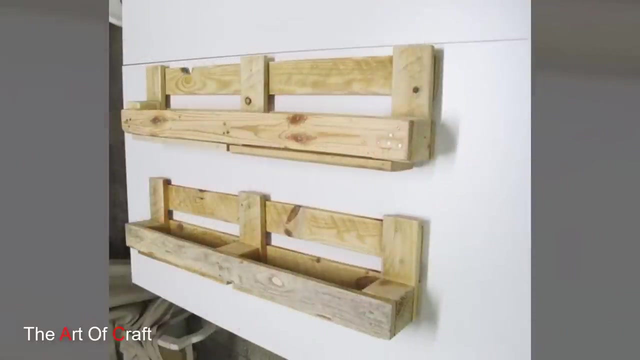 The inherent rustic charm of pallet wood allows for a wide range of designs, from shabby chic to industrial to modern minimalism. Customers can choose or commission pieces that match their unique taste and interior decor, making each purchase a personalized statement of style. 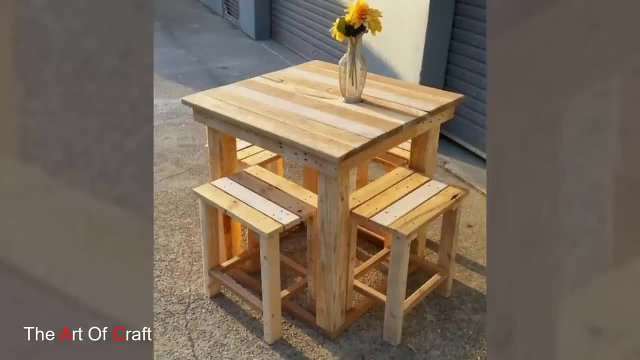 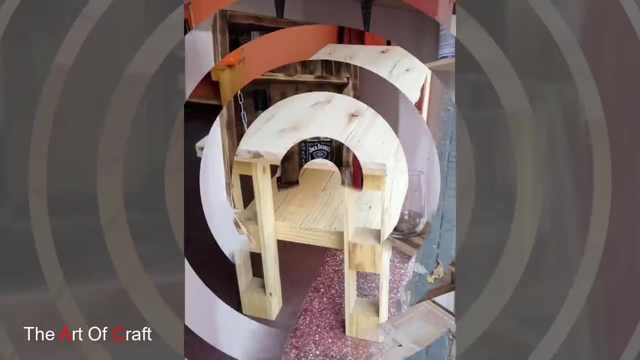 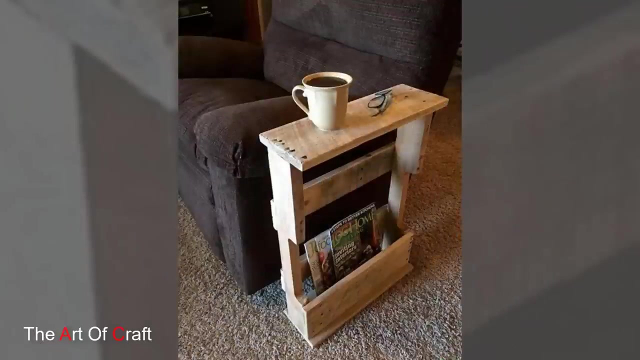 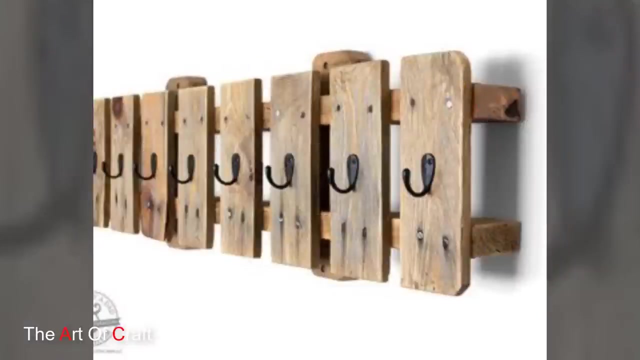 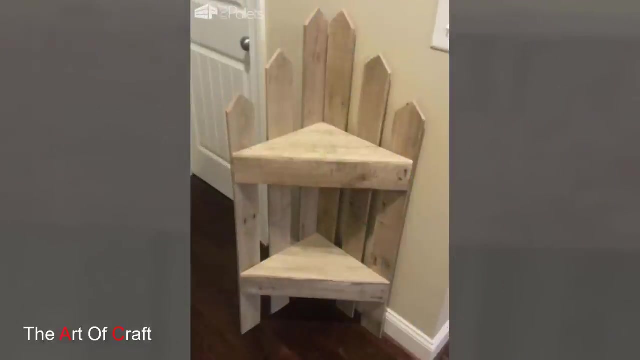 Compared to high-end designer furniture, Pallet furniture is often more affordable. The lower cost of materials and the DIY ethos of industry contribute to this cost advantage. Additionally, the widespread availability of wooded pallet means that aspiring entrepreneurs can easily source their materials. This accessibility allows small businesses and high-end designers to create their own. 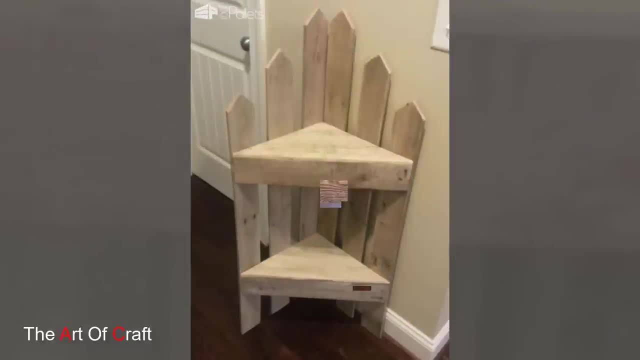 pallet furniture. Pallet furniture is also an art form. The allure of sustainability and eco-friendly options continues to grow. The allure of sustainability and eco-friendly options means that aspiring entrepreneurs can easily source their materials and materials that are well-experienced. The allure of sustainability and eco-friendly options can be used to build a good, artful. 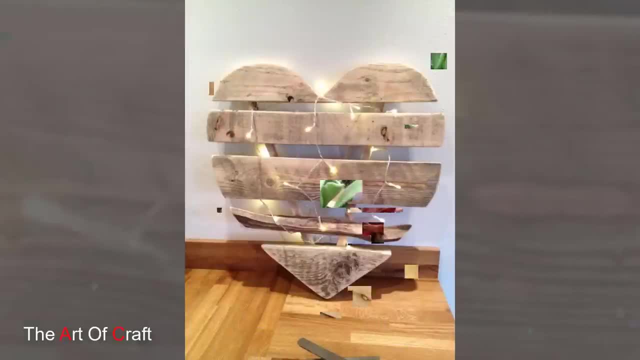 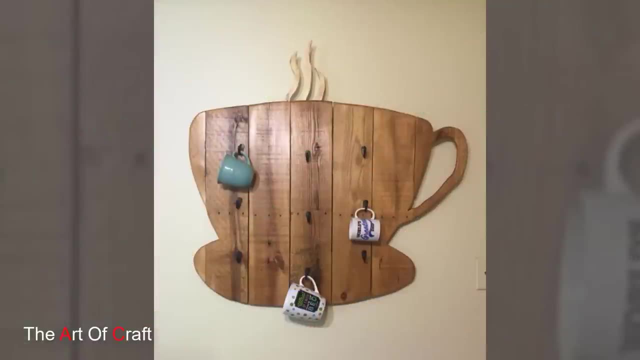 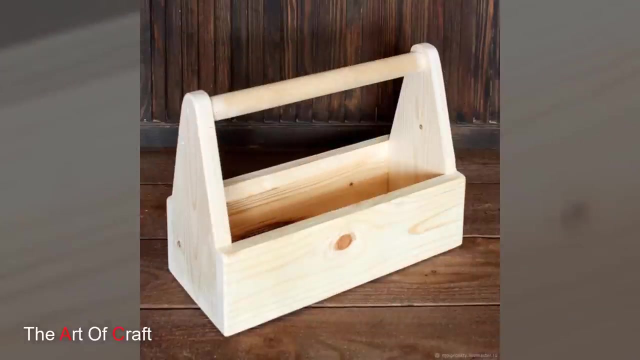 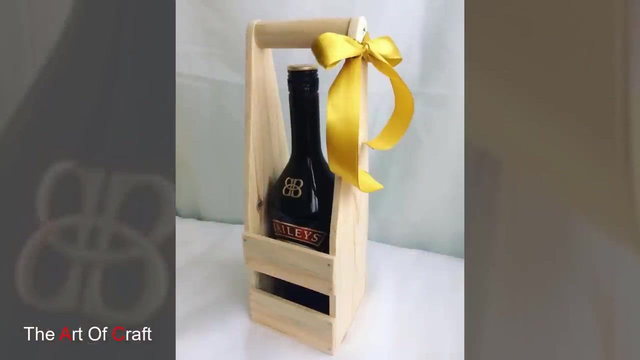 milling mill to create a high-quality, component-based, very luxurious business environment for their customers. Pallet furniture is a product of the Pallet's passion. The most popular sort of pallet furniture is the Pallet board. Pallet board is a sort of mini-pallet board. 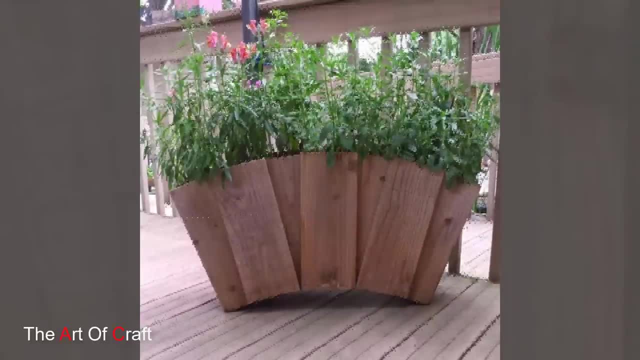 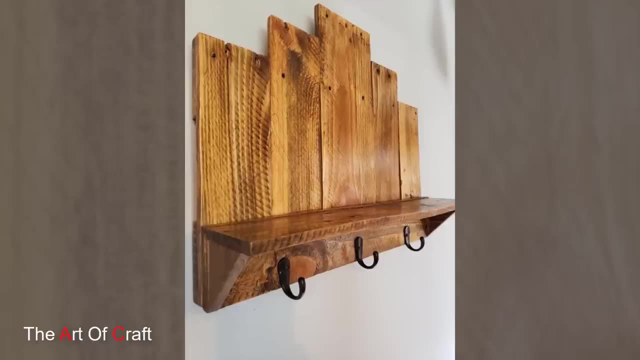 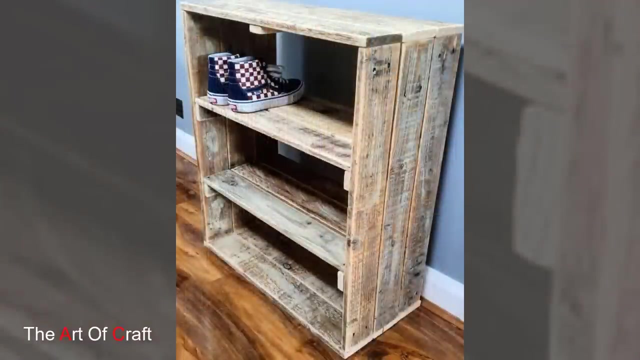 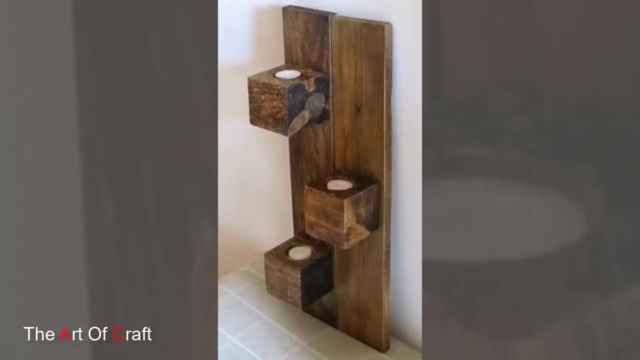 Pallet board is a more traditional type of wood. Innovation in market can be fierce, necessitating a strong brand and marketing strategy to stand out. Building a reputation for craftsmanship and reliability is crucial to success. The pallet furniture business is poised for continued growth as sustainability becomes an increasingly significant concern for consumers. 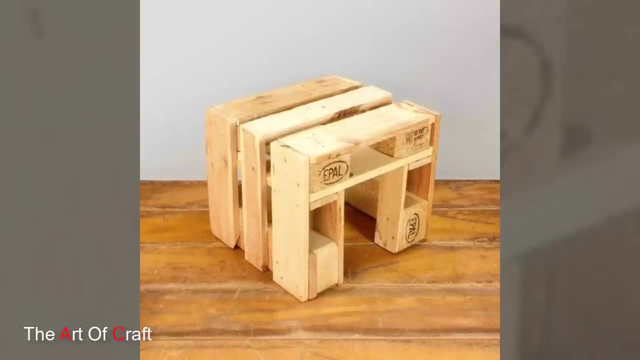 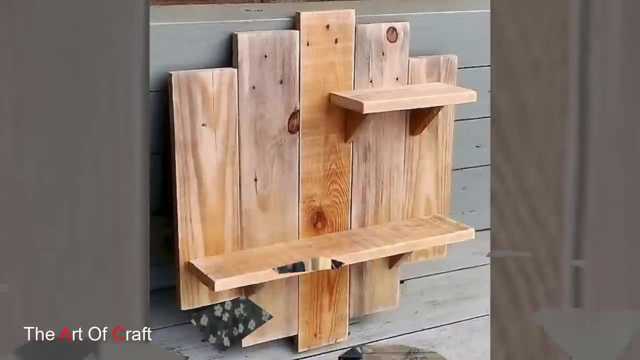 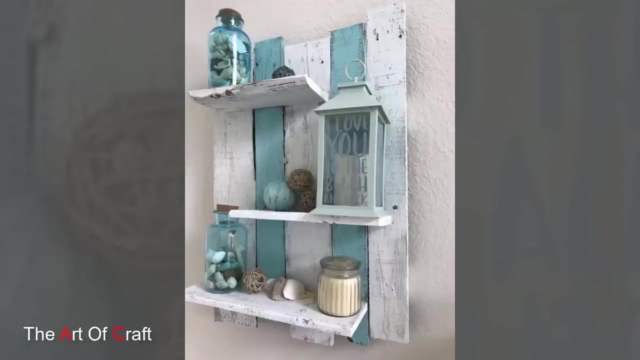 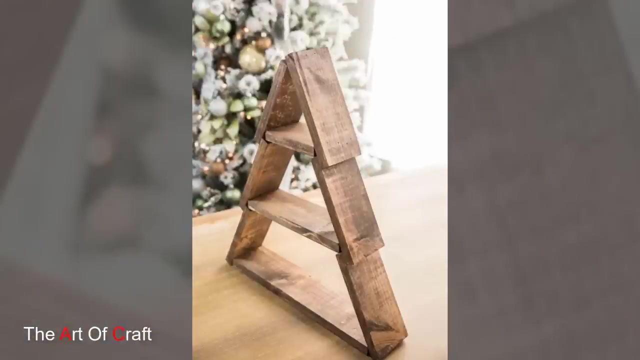 As people seek alternatives to disposable and environmentally harmful products, the appeal of furniture that repurposes waste materials will only intensify. Collaborations with interior designers and home decor influencers can also help expand the market reach. The pallet furniture business exemplifies the merit of sustainability. 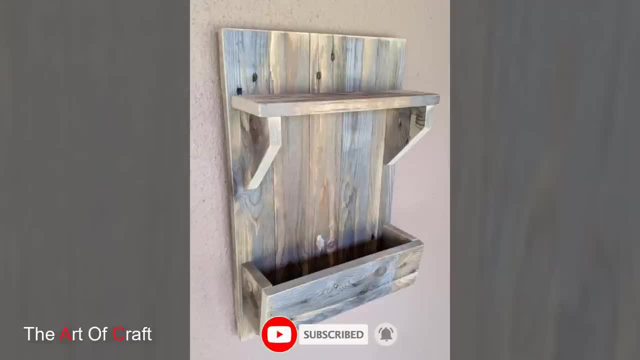 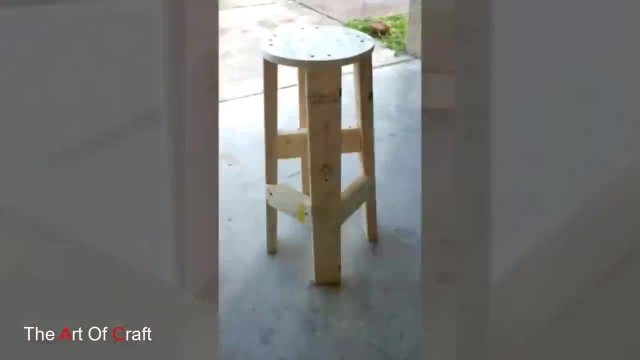 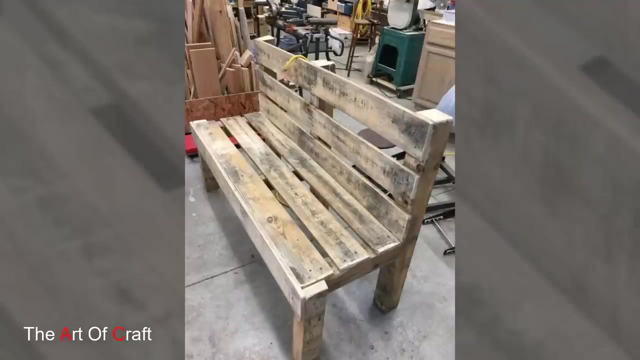 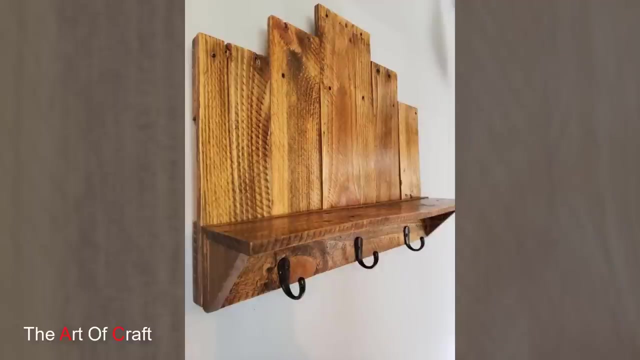 It offers eco-conscious consumers a chance to furnish their homes with distinctive handcrafted pieces, while supporting a more sustainable approach to consumption. As this industry continues to evolve and adapt to changing consumer preferences, it will likely remain a compelling option for both entrepreneurs and consumers alike. 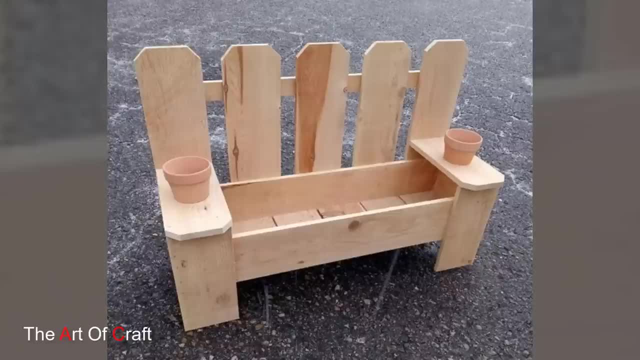 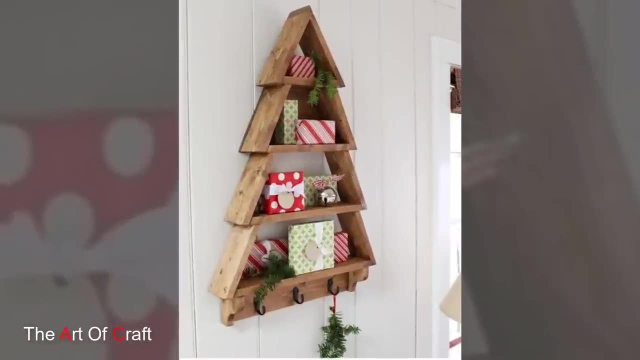 In the future, the pallet furniture business will continue to expand, seeking a greener and more aesthetically pleasing way to furnish their living spaces. I hope you were inspired to watch these ideas till the end. Which one of these ideas was your favorite? 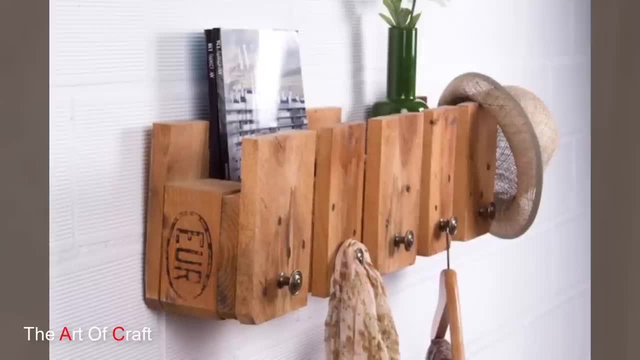 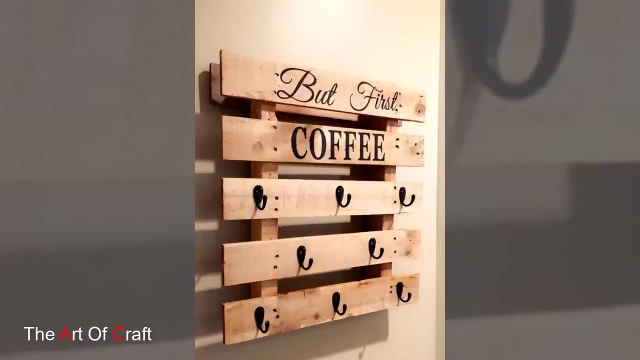 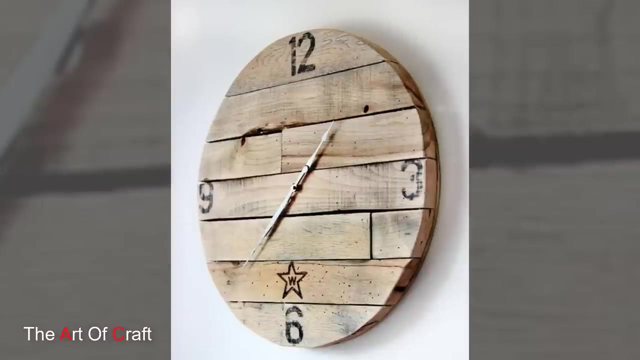 I would love to hear from you in the comments. If you would like to keep up to date with my latest videos about DIY projects, woodworking, metalworking, furniture ideas and more. You can subscribe us and click the bell icon for notification when we upload a new video to the channel.